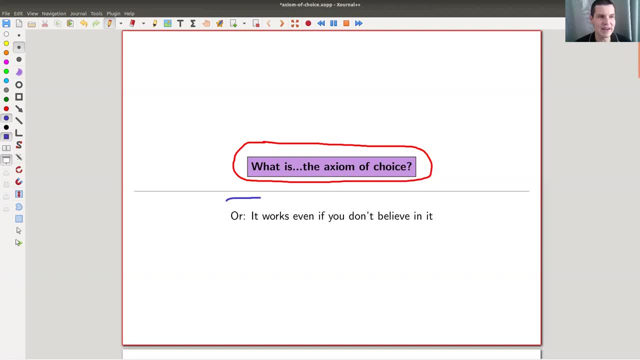 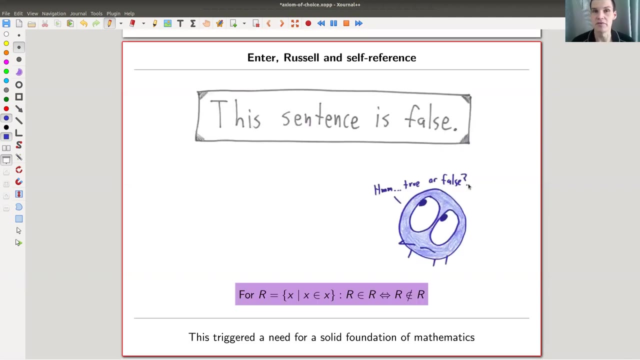 kind of can't do without. So I will take the following perspective. In the end you will see why I would claim it actually works, even if you don't believe in it. But before waffling too much so let's just get started with kind of the classical reason or the historical reason why. 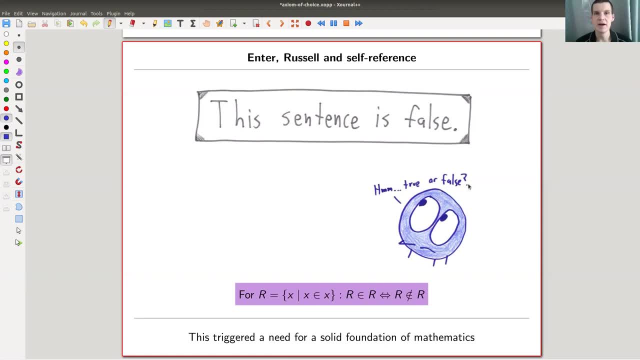 the axiom of choice actually came up in some sense. So everything is linked in the description In particular, there's a very nice page where I stole this picture from And it's really beautiful. It explains this idea of self-reference. Self-reference is always a problem Here, probably the most famous one. this sentence is false. 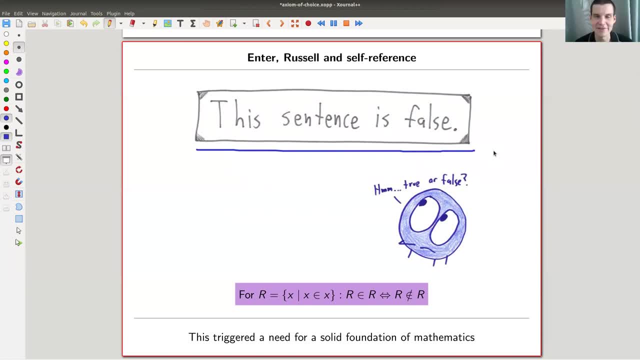 which is really a problem, because well, if it's true, then the sentence just says that it's false, And if it's false, then well, the sentence would be true. So is it true or false? We can't really. 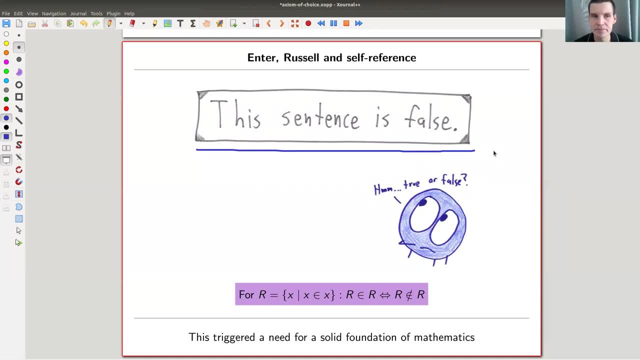 tell. So you're always run into problems. If you could formulate those self-reference paradoxes- and there are zillions of those in classical language, in just our language, everyday language- if you could formulate them in some logical system in one way or the other you run into a problem, And it's always kind of the same idea. So all of 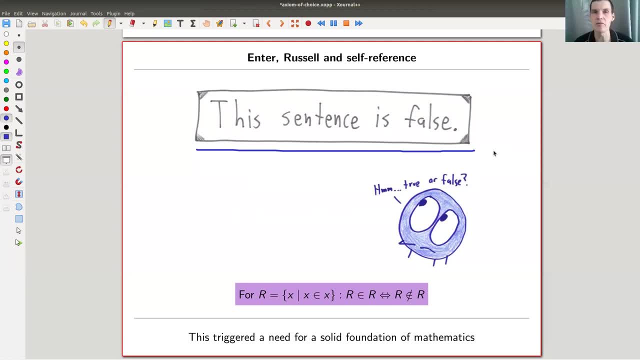 these things like Lagoon's incomplete theorem. in the end it formulates the sentence in some form in a system containing certain types of logic, so not a certain logical system, And this just kind of means that this sentence cannot be proven from. 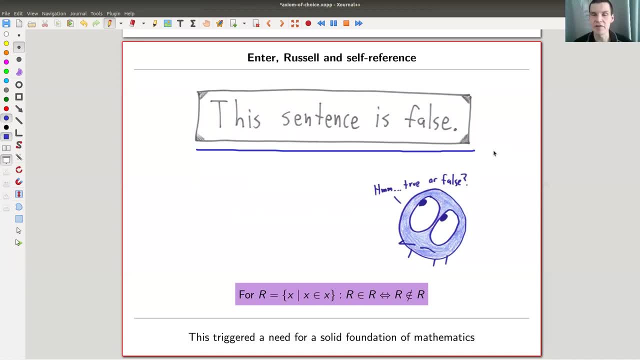 your system of logic. Another example in everyday language is, for example, I am lying And well, have I just said the truth or not? If I have said the truth, then I was lying. If I was lying, then I have said the truth. So in everyday language you will find zillions of examples. 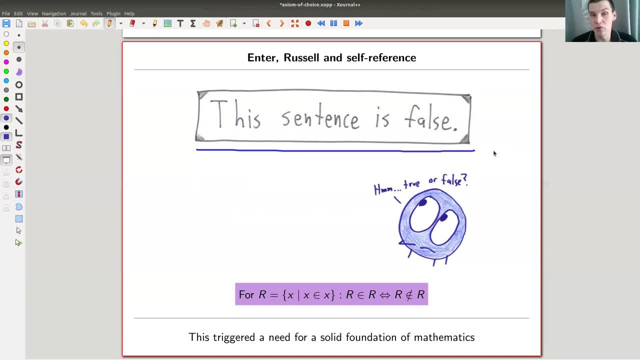 And, as I said, the main problem is, or the main problem from the viewpoint of logic, mathematics and philosophy is, if you kind of face that sentence like this sentence is false in your favorite logic system. And Russell did exactly that. He found a version of self-reference of the sentence false. 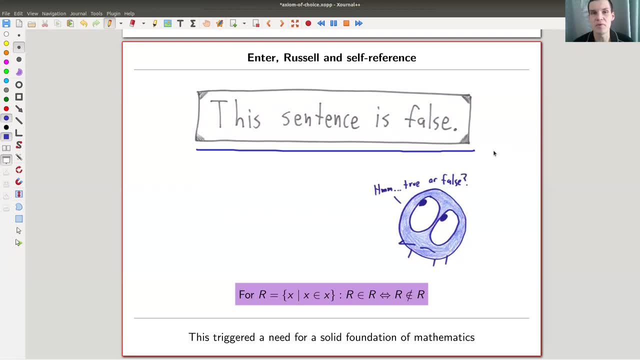 in set theory. And set theory something like 130 years ago was kind of everyone wanted to be kind of the foundations of mathematics And it's kind of a problem. So what Russell did is written here. So if you take a set and you call it r, r, like Russell, and it's defined by it contains all x. 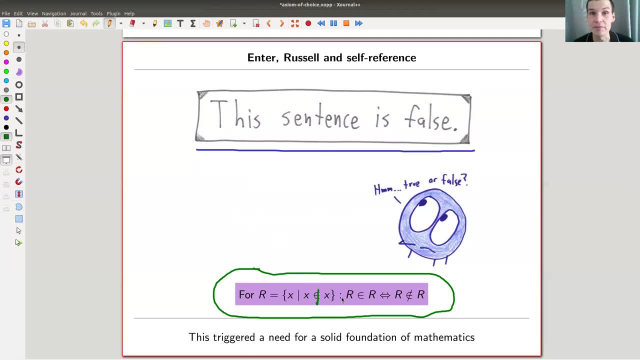 which do not contain z themselves, though it should be a do not contain themselves here. then you might wonder: what about the set R itself? Is it in itself or is it not in itself? Well, if it is in itself, by construction. 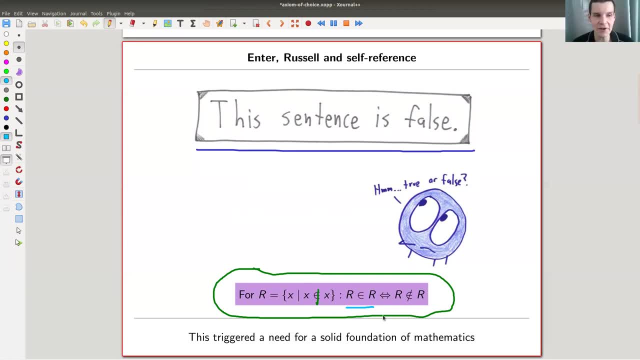 of the set R, it's not in itself. And if it's not in itself it is in itself, And this is a really classical example of self-reference. The set is kind of referring to itself, And that's a problem. It always causes a problem. So we now have a kind of a contradiction here. This set kind of can't. 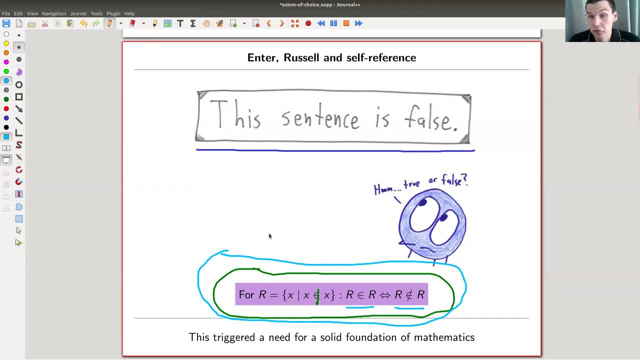 exist. It is contained in itself And at the same time it's not contained in itself. It's a huge problem if you want to build foundations of mathematics. As I just said, if you have the sentence is false in one way or the other in your system of logic, you are kind of dead. You don't. 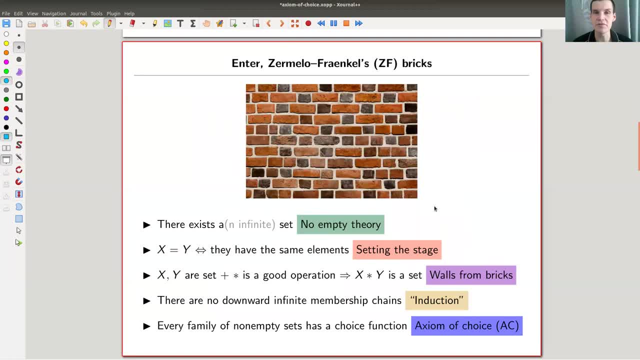 want that And people start to think about how to solve that, or let's say how to kick out the set R of our set of axioms. And there are many approaches to do that. The most popular one is whatever I call it, ZF. It's a Melo-Fraenkel approach. There are different ones linked in the description. 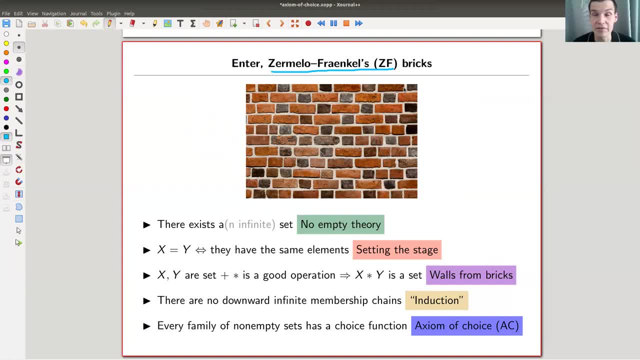 You do not even need to use set theory. There are already different axiom sets for set theory. You don't need to do that. You can do type theory, homotopic type theory, topoid theory, category theory. You could throw a lot of axiom systems on your foundations of mathematics. This is certainly 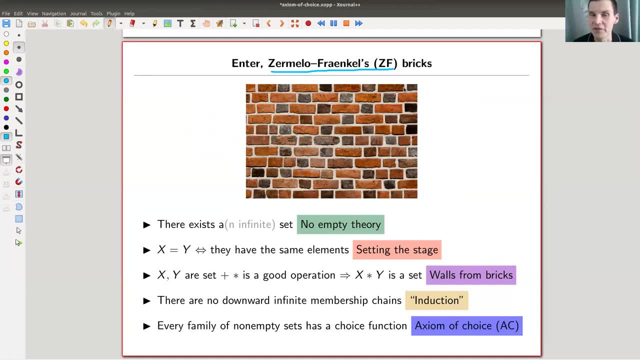 the most famous one, And I kind of don't want to discuss the question whether you should believe in one or the other, because it's kind of a matter of taste anyway. So let me rather try to explain this same Melo-Fraenkel set theory without writing down the axioms. 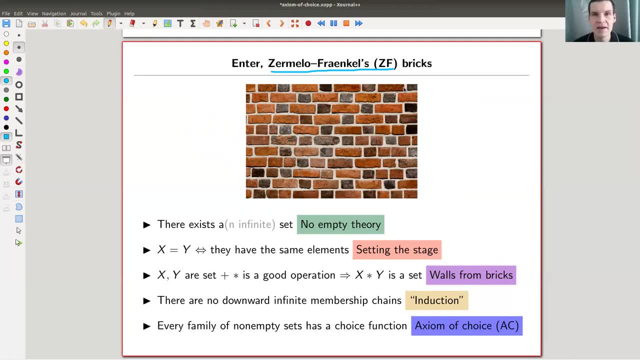 because, well, there are nine axioms-ish And they all read. well, they are formulated in its formal logic, of course. That's the whole point. So they all read a little bit strange-ish. Let me just explain the main strategy here. So the main strategy: how to avoid this paradox due to Russell. 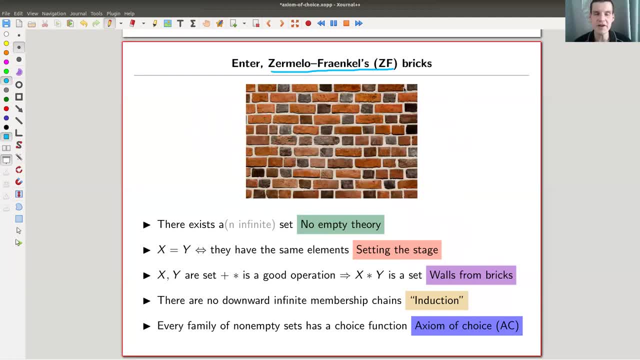 or this funny set R. So what they do is they kind of try to build sets. So what they do is they try to build a set theory using this picture in mind: Like I give you a certain number of bricks and whatever you can build from those bricks, that's a set. That's. 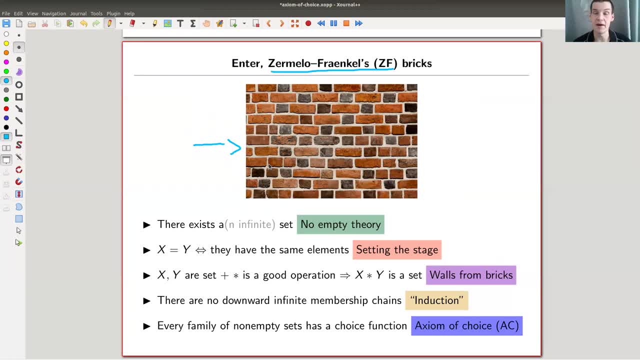 the approach A little bit more formally is the axioms. one of the first axioms says that there is some set. okay, Sometimes it says there's some infinite set. depends a little bit on your taste, Anyway. so there is some set And that's just. I mean, yeah sure, I accept that If you want to. build a theory on sets, then that's fine. But if you want to build a theory on sets, then that's fine. But if you want to build a theory on sets, then that's fine. But if you want to build a theory on sets, 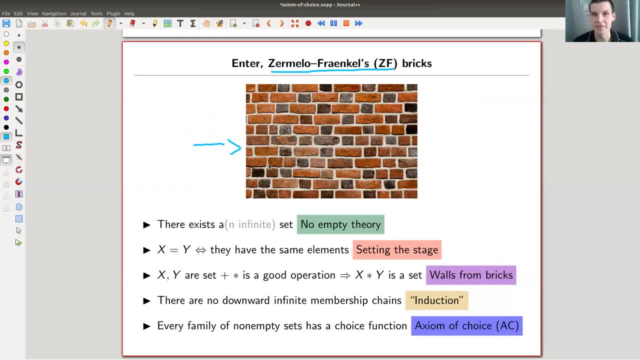 then I should kind of assume the existence of at least one set That's an axiom. There exists a set that's an axiom, something you can't prove from more fundamental principles. So this is kind of okay. I would give it. I think it's kind of okay. The second one is roughly of this form You want. 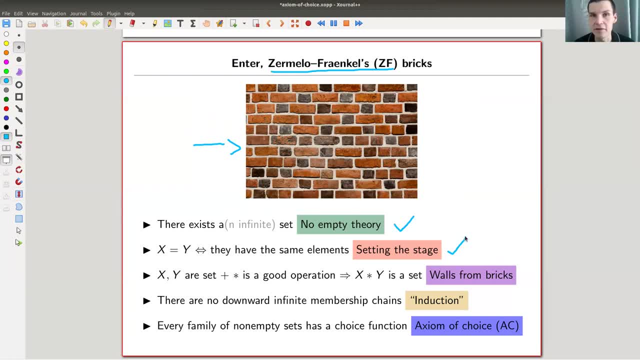 to define a notion of equal, And in the set theory it's: two things are equal if they have the same elements. I kind of also accept that one. And then comes the main strategy that they proposed, And I kind of also accept this one, which is basically saying: you have a set, you have another set, you. 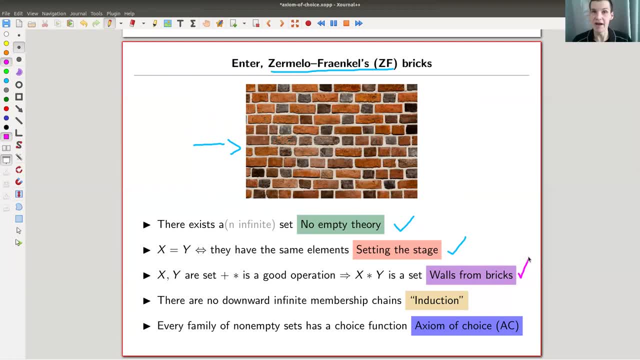 have an operation that you like, for example taking union, and whatever you do gives you another set right. It's this brick principle: You have a brick, you have another brick, put them together, you get already a piece of a wall and you can use it then again to build bigger walls. 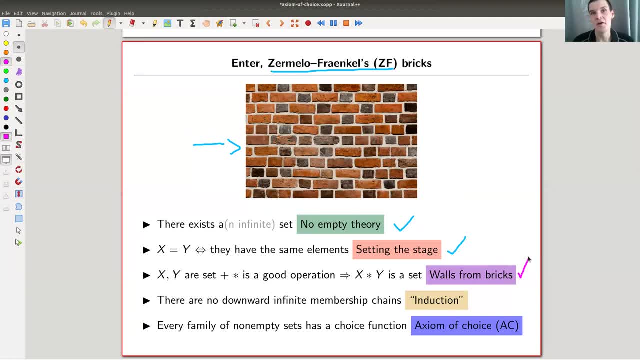 That's this idea of using bricks And that kind of throws out the Russell set, because in the end it turns out that the Russell set is just not a set, right? So how do you solve the question whether this statement is false, is true or false? Well, you ignore it. You just throw out the 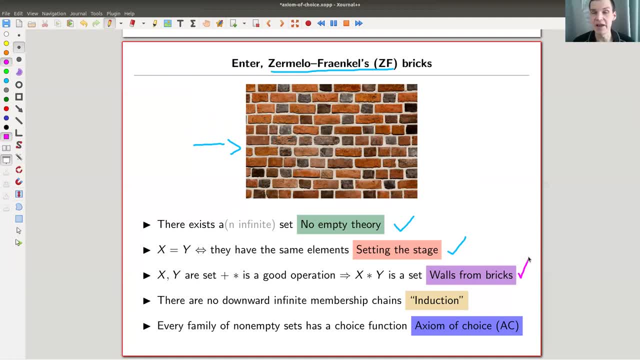 question. There is no yes or no statement related to this statement is false. You just kick it out of your logic. It's not provable, It's not accepted in your logic And you kind of do the same here in this brick type fashion. Okay, I kind of kind of do accept that. And then there's a slightly funny sounding axiom. You kind of do the same here in this brick type fashion. Okay, I kind of kind of do accept that, And then there's a slightly funny sounding axiom. You kind of kind of do accept that, And then there's a slightly funny sounding axiom, But in the end it's. 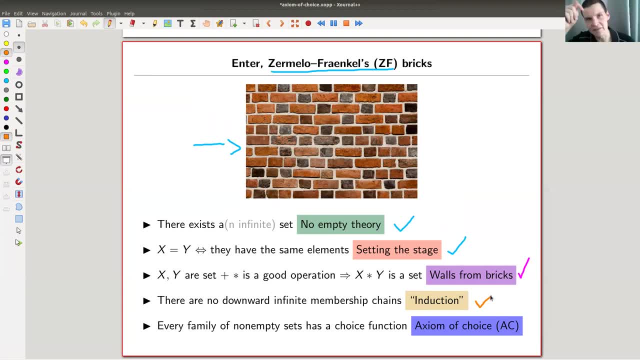 it's a form of induction. It's not quite link is in the description. It's called the axiom of foundation, but it's kind of an induction thing. So mathematical induction is a very powerful tool In some sense. you can't produce that from simple axioms, So you just put it in your back of axioms. 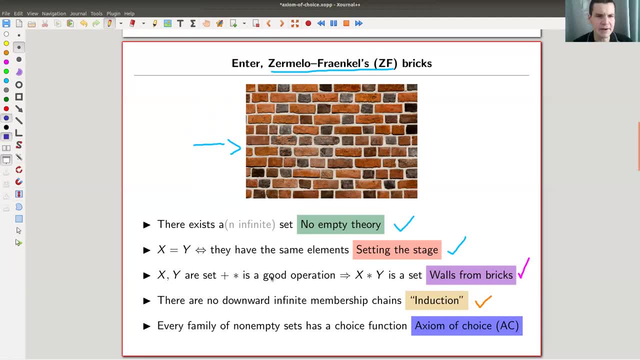 And yes, I would like to accept that. And then there's a slightly funny thing which is the axiom of choice, And we are not really sure whether we want to accept it or not. Roughly speaking, it just is the axiom of choice And we are not really sure whether we want to accept it or not. 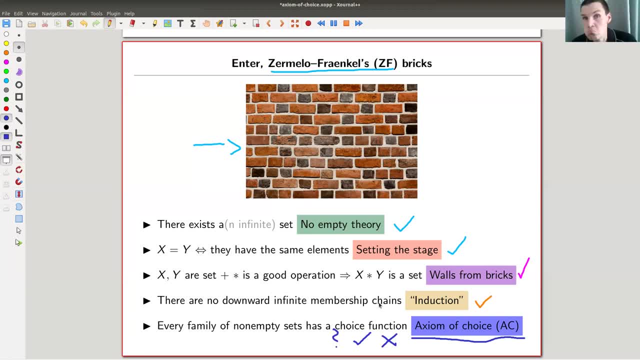 Okay, It sounds harmless, but let's go into some details here. So what I want to try to say on this page is: there's this strategy to throw out the paradox given by this statement is false, by using a brick principle and all kind of axioms that you throw into this. 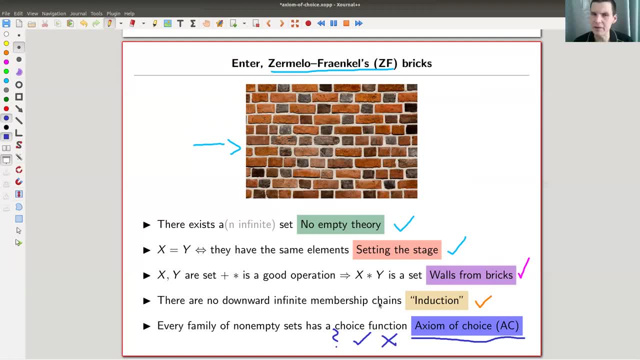 back of axioms are kind of okay, kind of believable, acceptable. And then there's one that sounds a little bit strange, So let's have a look at this one. And then there's one that sounds a little bit strange, So let's have a look at this one. 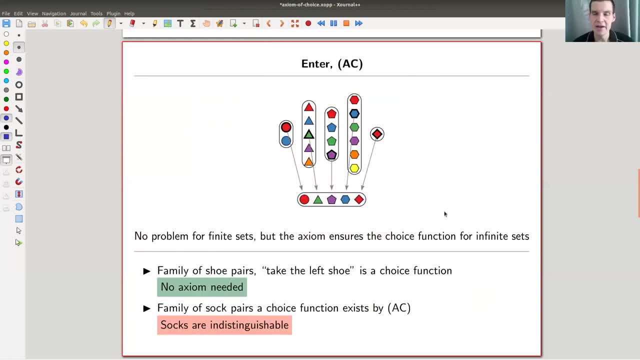 the axiom of choice AC in the notation for today, And it's actually a pretty simple statement. It's what I've illustrated here above. So you have a certain type of families of sets- In this case you have five- And then there's a choice function. 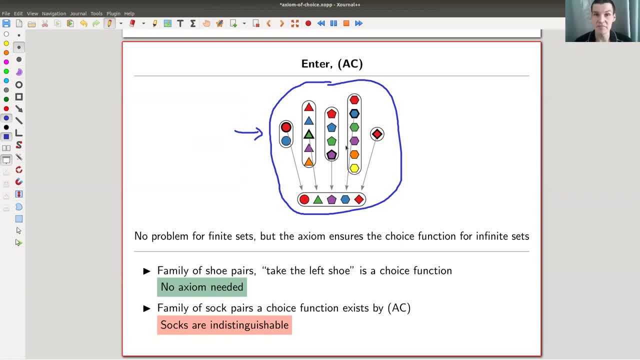 which is, you pick out one element from each set. Sounds pretty harmless, but let's think about two examples. So, for example, you can have an infinite number of shoes or pairs of shoes, set an infinite number of them, whatever. 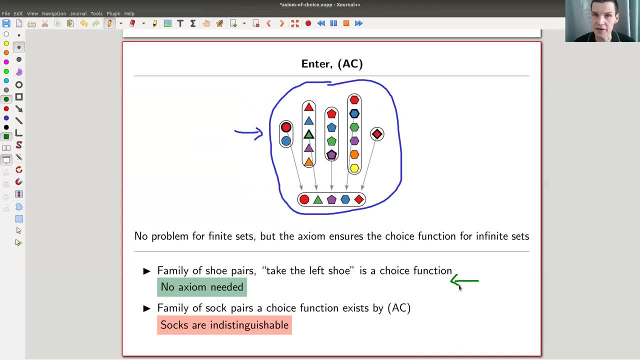 And the question is: can you produce a choice function Meaning, can you produce a rule in some sense such that everyone would pick the same shoe out of each set, right? I have a lot of sets containing shoe and another shoe, and I have more of them and I have infinitely many of them. 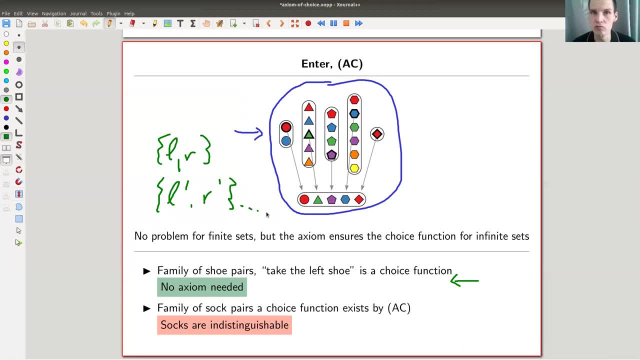 And the question is: can I tell you a rule such that both of us would pick the same shoe? And yes, I can. I can say something like: yeah, please take the left shoe. That's a rule. So we have an infinite number of sets. 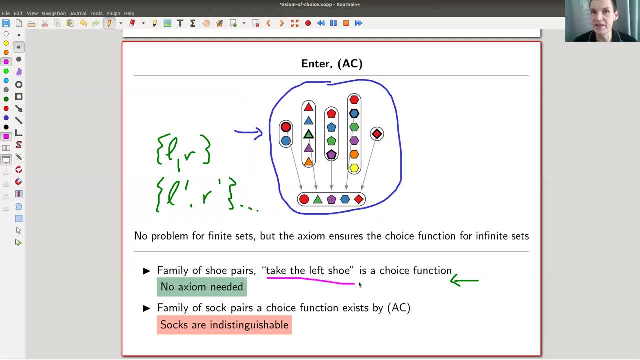 But I gave you a rule, so I gave you a choice function without actually needing that axiom. right, The axiom proposes the existence of the choice function, But for some sets that's actually needed. So, for example, if I would replace my shoes, 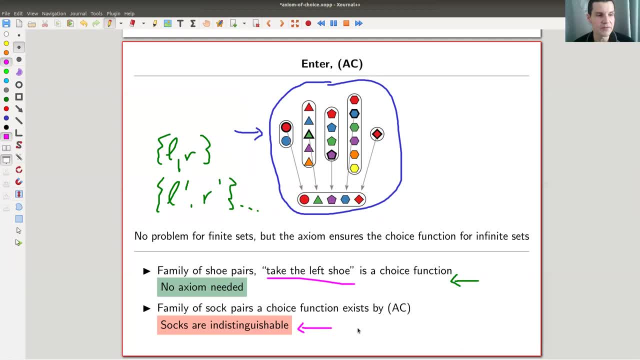 so this example is due to Russell. So if you replace shoes with socks and you kind of assume that socks are indistinguishable, and now you have again pairs of socks, a lot of them, but you can't really tell the difference, which one is which. 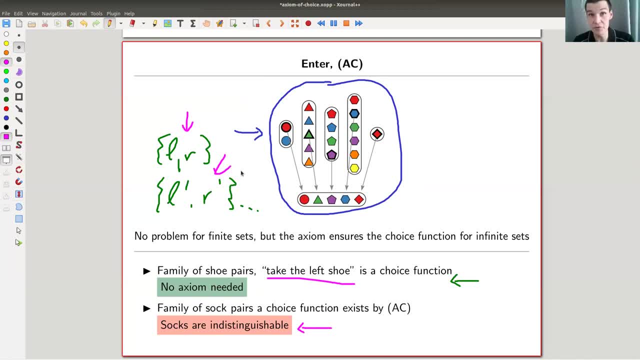 can you still produce a choice function such that me and you pick the same sock out of each set? That's less clear. Why should that work? Not quite clear, But the axiom proposes that, yes, this works, And that makes it already a little bit fishy, right? 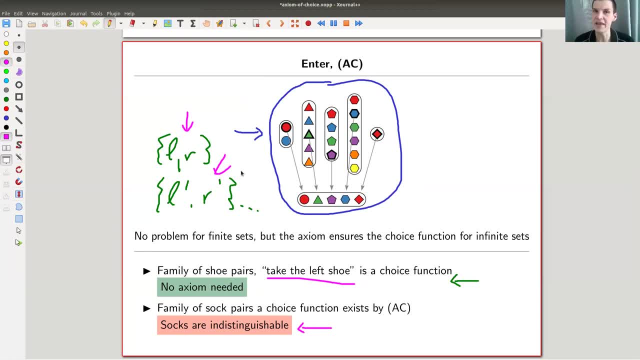 It's. It's not like the other axioms. The other axioms are fairly harmless, Like if I have a set, I have another set, then the union is a set. That sounds pretty harmless to me. This one is a bit fishy. 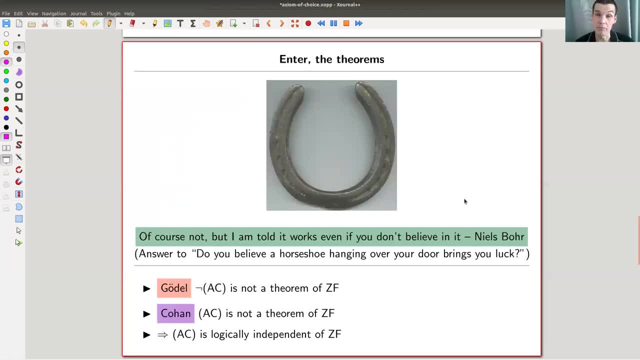 Turns out- and here's the theorem that Gödel proved- that you can not prove not AC. very complicated, So not AC is not a theorem in Tamela, Frankel's set theory, So you can't prove it from the other axioms. 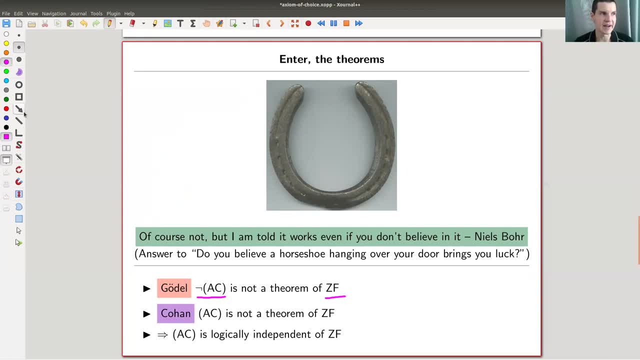 You really need to throw it in if you want it. On the other hand, the statement due to Cohen, which was much later, it kind of says the opposite. So you can also throw in, not AC, if you want. In other words, this axiom is really independent of the other axioms. 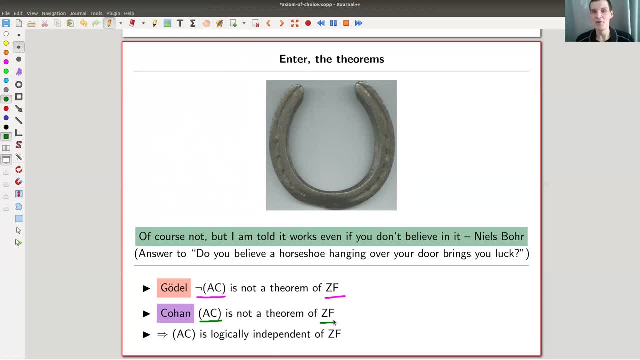 And it's kind of your preferred choice axiom of choice, if you want, whether you take it or not, In some sense it's kind of a weird statement. That's a really nice theorem: independence. So this is my theorem for today: independence of the axiom of choice. 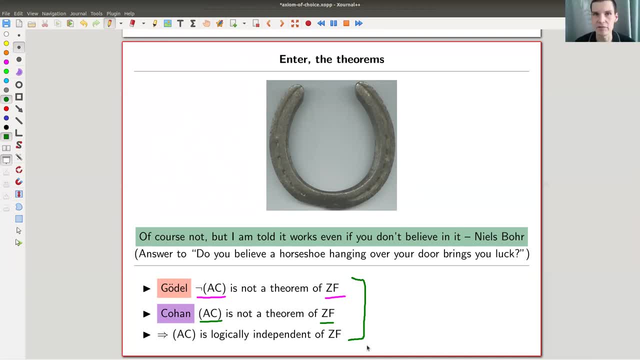 This is fine, This is a funny axiom And it's actually independent of the other axioms, Kind of a fun statement And I would really like to take- we'll see it on the next slide- a little bit in more details. I would really like to take this approach of Niels Bohr. 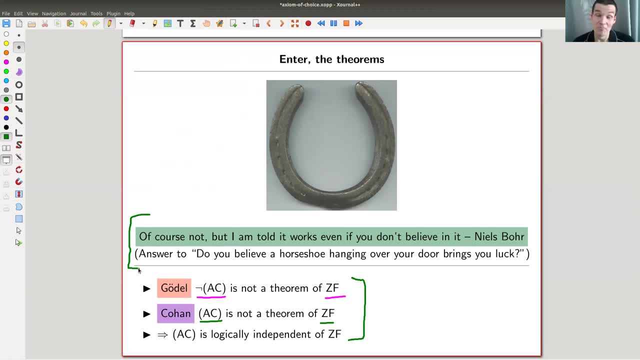 Of course Niels Bohr, very famous physicist. Let me just quote Niels Bohr. Of course not. Of course not, Come on, Of course not. But I'm told it works, even if you don't believe in it. 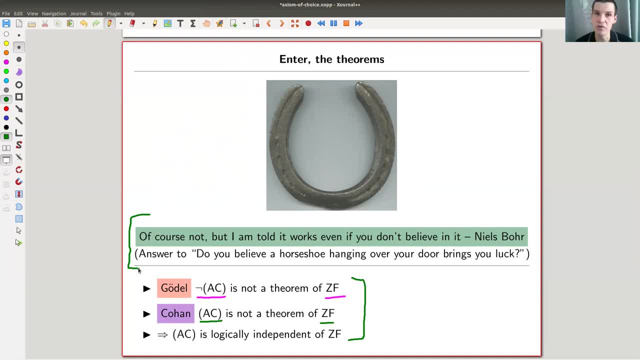 And this was the quotation. just answer to the question: Do you believe a horseshoe brings you luck or not? But Niels Bohr just says: of course, I don't, Of course not Come on, But if it works, then it works anyway. 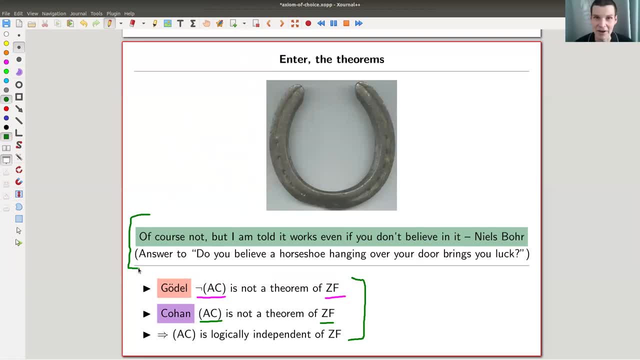 That's kind of the approach, my approach to the axiom of choice as well. So in some days, yeah, I would take it, On some days I wouldn't. And it's independent anyway. So it doesn't matter whether I believe it's true or not. 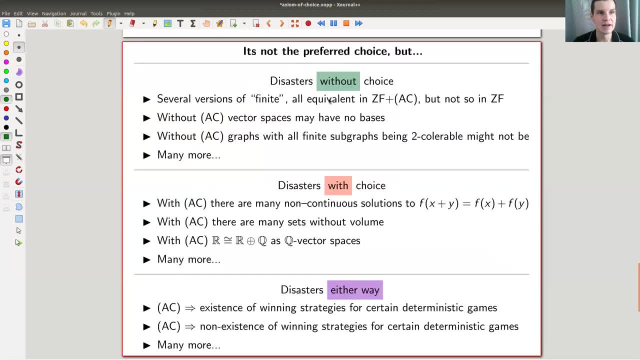 It actually doesn't matter. And let me finish by telling you a little bit why it's this axiom of choice. It's so controversial. I mean, I kind of sketched it with my shoe and sock example, But still, you can still believe that, well, socks are pretty nice sets of socks. 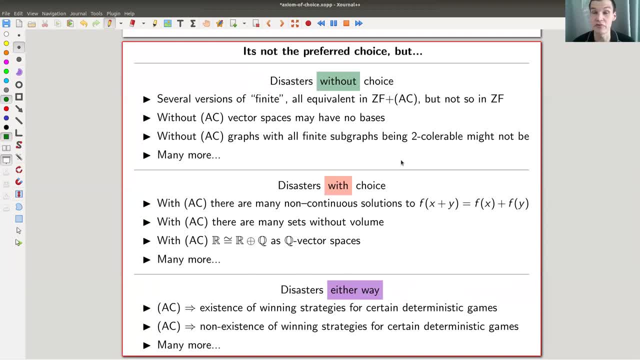 Well, who cares? And of course you can assume the existence of a choice function. Why not? But turns out the choice is much more delicate in mathematics. So in the beautiful book Axiom of Choice by Herrlich, linked in the description there, 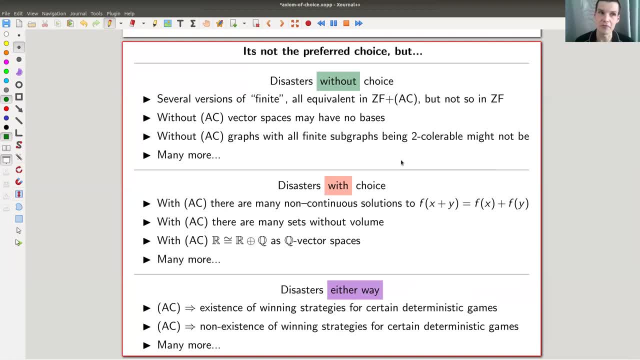 are basically three chapters. There are more chapters, but there are three- And one of them is called disasters without choice, One of them is called disasters with choice And one of them is called disasters either way. So it kind of doesn't matter. 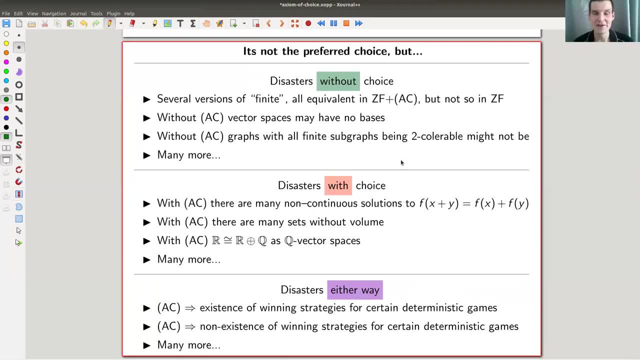 Take Neil's boss approach, It kind of doesn't matter, You run into trouble either way in some sense. So let me discuss some of them. So for example, if you would? we now know choice is independent, So it's a matter of taste whether I want to take it into my axiom system or not. 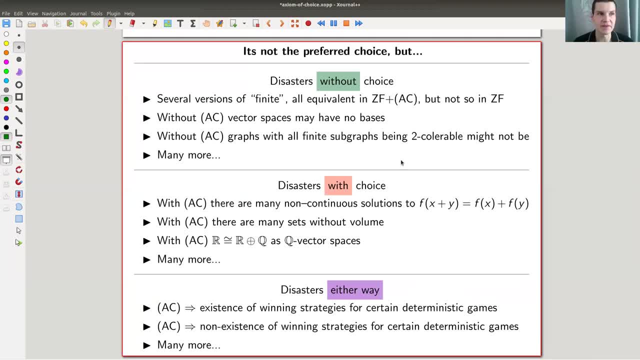 If you don't want it, then you get something like: the notion of finite is not quite clear anymore And there are several approaches to that And all of them are equivalent as soon as you have that choice, But if you don't, then they're actually different, which is kind of a weird thing. 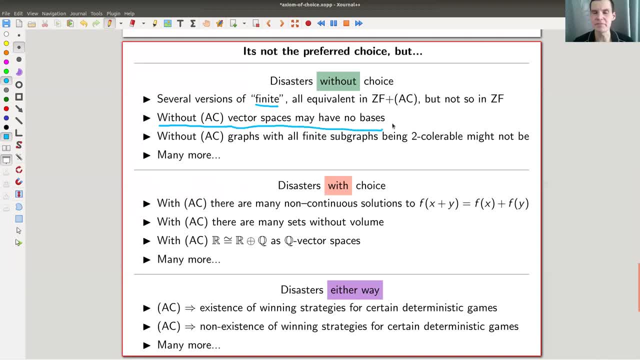 If you're more like an algebra type of person like me, then you get something like vector spaces might not have bases, which is really bad in practice. right, Vector spaces resolve bases. That's really bad. And you also get statements in graph theory, for example, something like: you can have a: 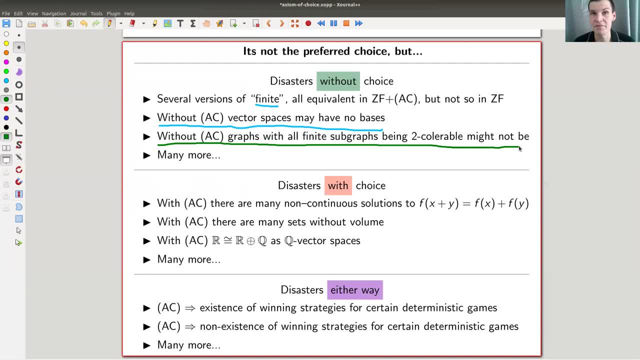 graph such that all finite subgraphs can be colored with two colors, but the graph itself can't, which is also a bit strange. So you have several disasters turning up in various parts of mathematics. I could make this much longer. The real numbers are always very good. 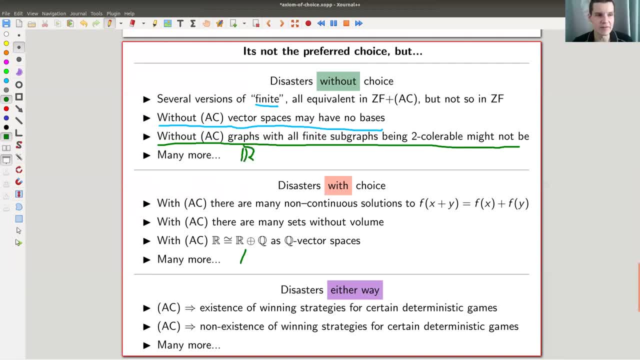 There are a lot of disasters appearing in the real numbers And here as well, of course. here we'll see the real numbers in a second. a lot of disasters and more in analysis and so on. So if you don't want the axiom of choice, you run into those problems. 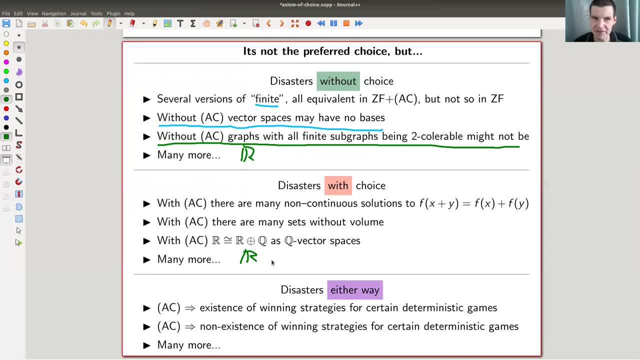 OK, Then you might say, OK, maybe it's not so bad, Maybe let's accept it, But you will run into other problems, So there's just no way out. So here are some disasters with choice, So probably the most famous one is the existence of non-measurable sets, strictly speaking. 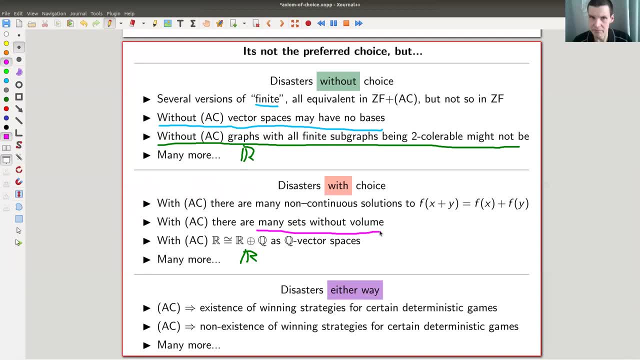 is some of them. Some of these are not equivalent to the axiom of choice, But anyway, let's ignore that So you can have sets without volume. That's already kind of strange. You're going to have non-measurable sets And, as usual, if you have one of them, you have many of them, really many of them. 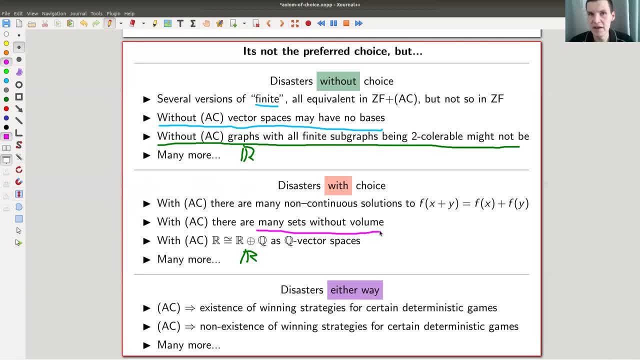 So this is already kind of strange. So if you accept the axiom of choice, you accept the existence of those sets. basically, One for more kind of classical analysis would be this harmless-looking equation: here, which is like a linear equation, I can have non-continuous solutions. 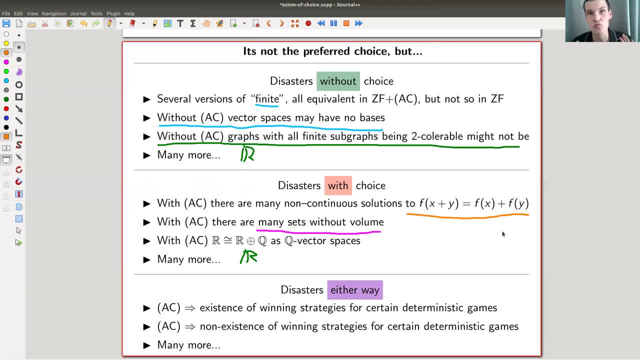 And as soon as you have one of them, you have many of them. That's kind of a weird statement. anyway, Here's one from algebra again if you want. So r and r plus q are actually equivalent as q back to space, which is kind of weird. 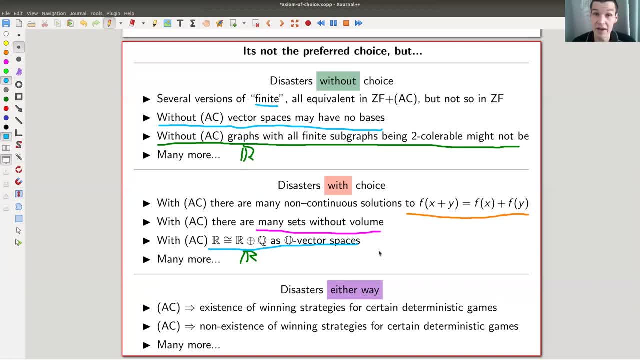 And there are many, many more, many, many more statements that you get disasters, that you get with options, And there are also disasters either way. So really I take Neil's boss approach. So, for example, in game theory, you can construct certain deterministic games which have winning.